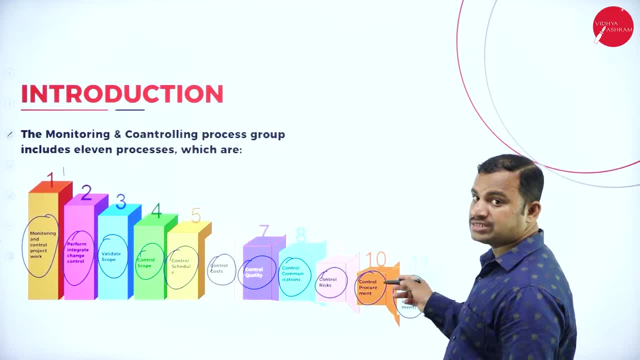 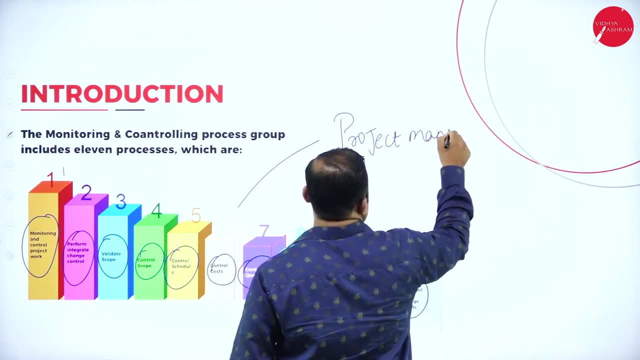 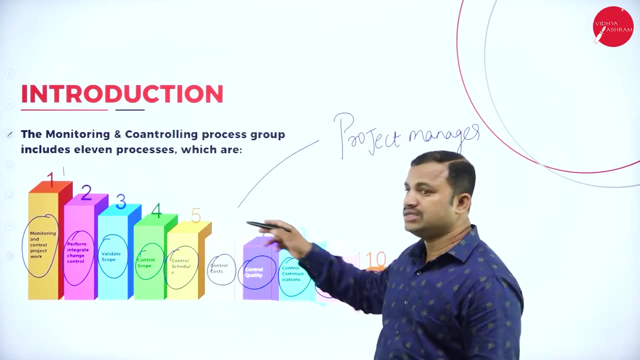 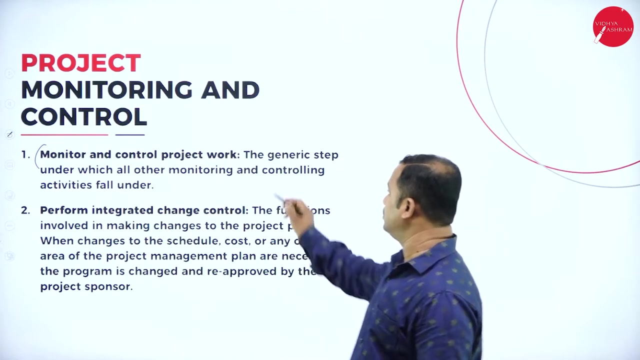 stakeholders. all these are different types of activities that are monitored by the project manager, that is, project management is a skill that helps them to control all these activities, for example, monitor and control project work. what is the meaning of this? the generic step under which all the monitoring and 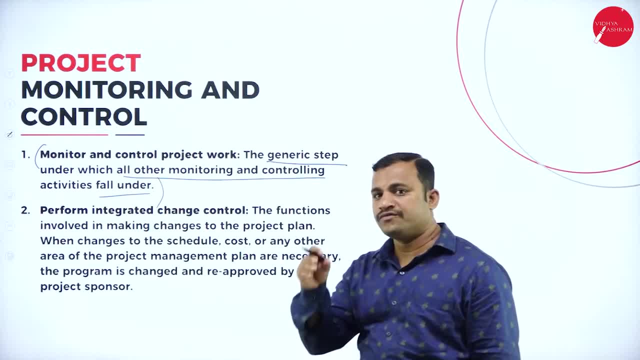 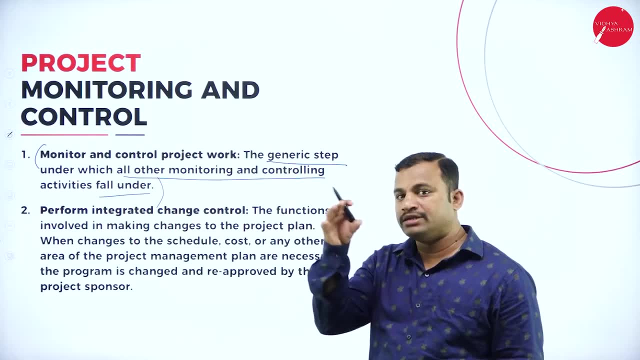 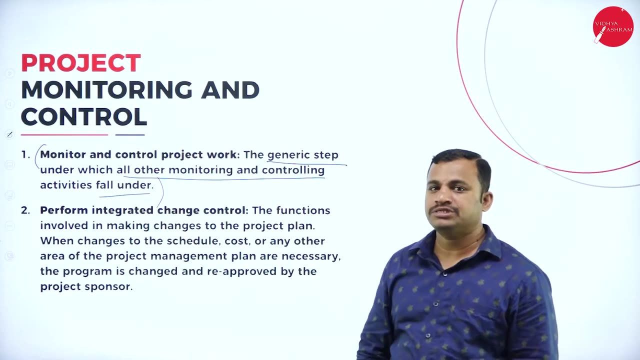 controlling activities fall under. that means whether all of the team members are doing their tasks assigned to them properly is monitored by the team leader. whether team leader is getting the results properly from the team members and given to the project manager. what is the progress of that? all those things? 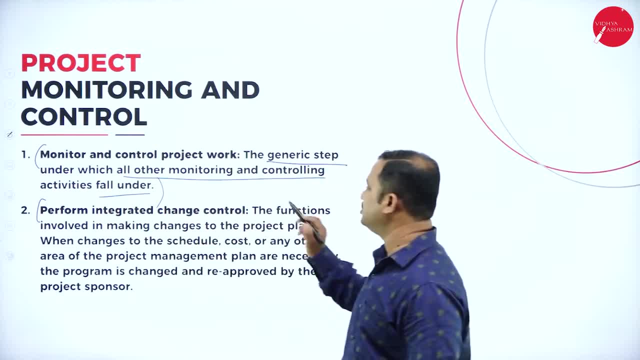 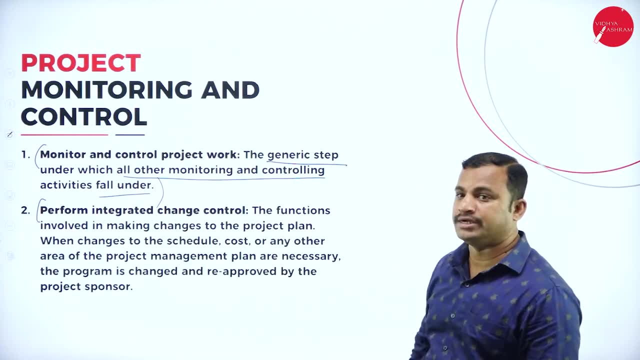 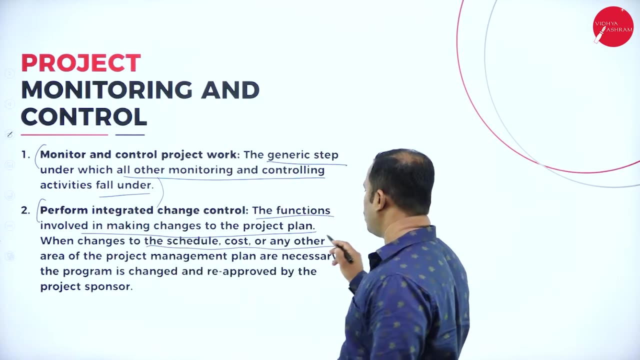 are monitored here, then perform integrated changes control. that means once all these modules from different team members are integrated together, it has to be monitored. then the functions involved in making changes in the project plan, when changes to the schedule, cost or any other area of the project management plan are necessary. 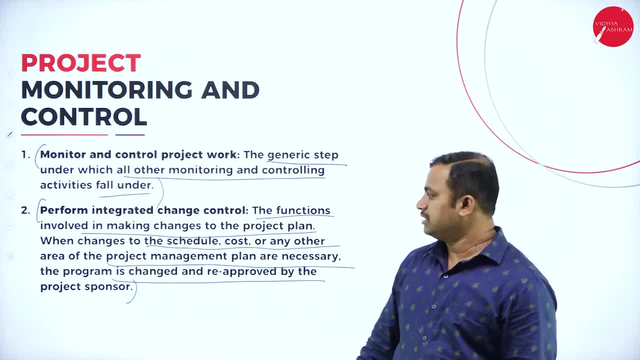 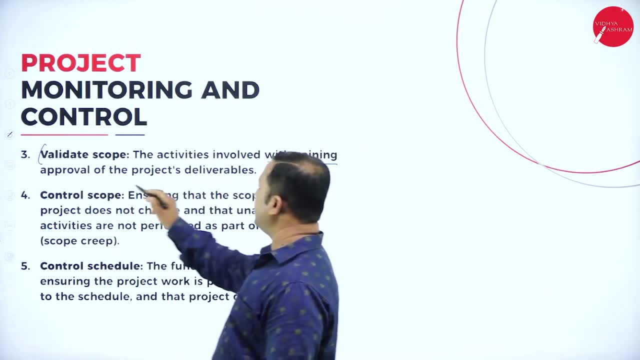 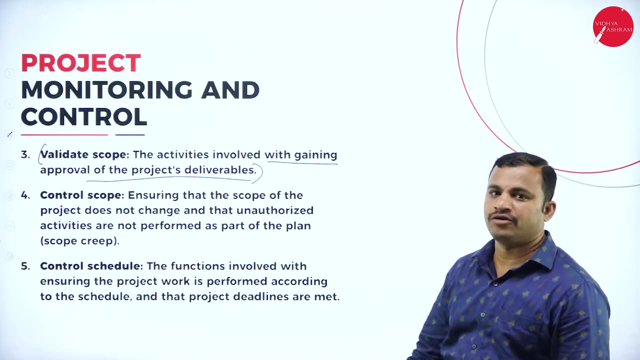 the program is changed and re-approved by the project sponsor. that means it has to be done by the project manager, then validate scope, the activities involved with gaining the approval of the project's deliverables, which are the different types of deliverables we deliver to the client, that is, the software product, user manuals and 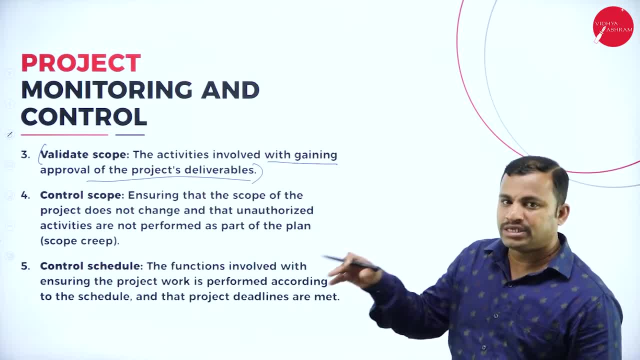 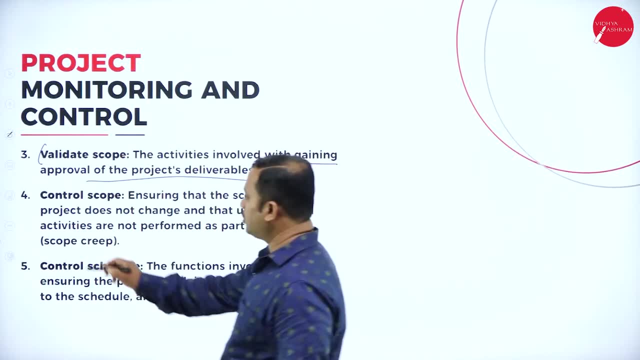 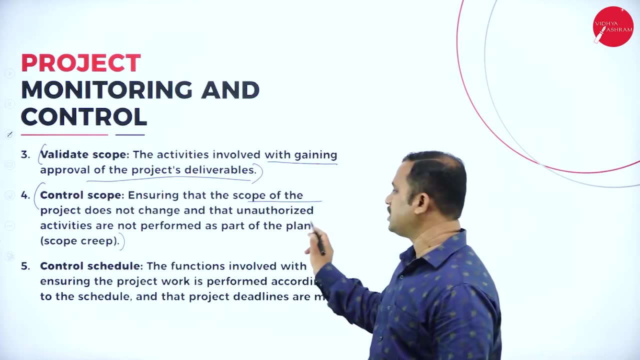 the software which are dependent on the executable code. all those things are delivered to him and it has to be validated. control scope: this includes ensuring that the scope of the project does not change, that the unauthorized activities are not performed as part of the plan. that is scope creep, then control schedule. that means the timing specified time. 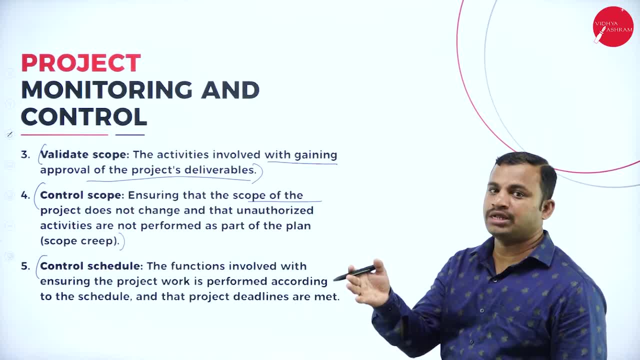 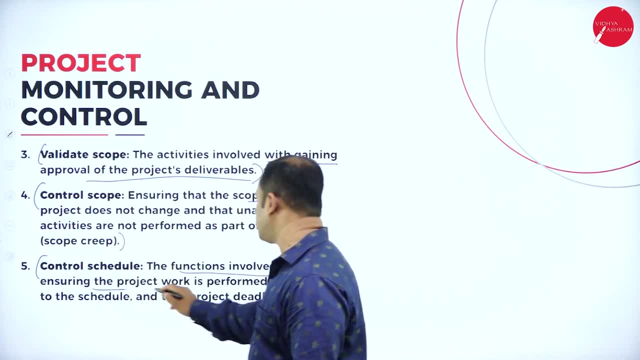 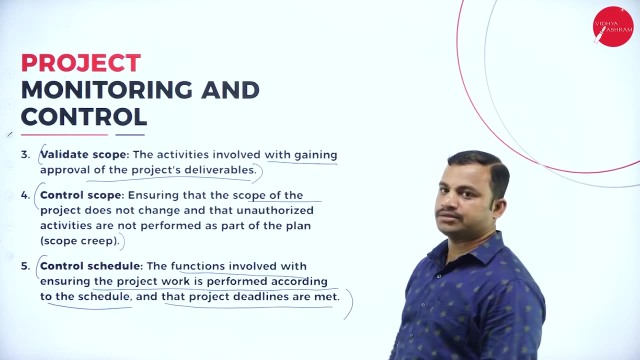 limit is given to the team members as well as to the team leader. they have to follow the instructions carefully. that means the functions involved with ensuring the project work is performed according to the schedule, that is, the time given to them time limit, and that project deadline are met within the 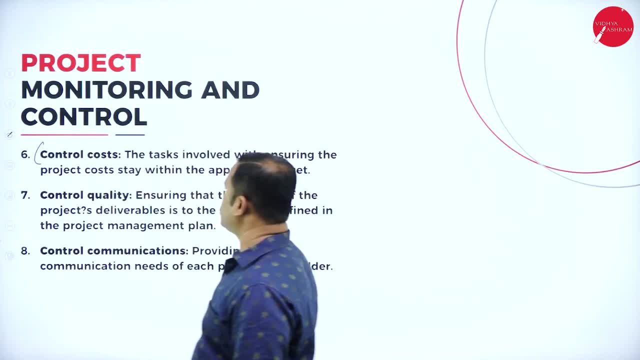 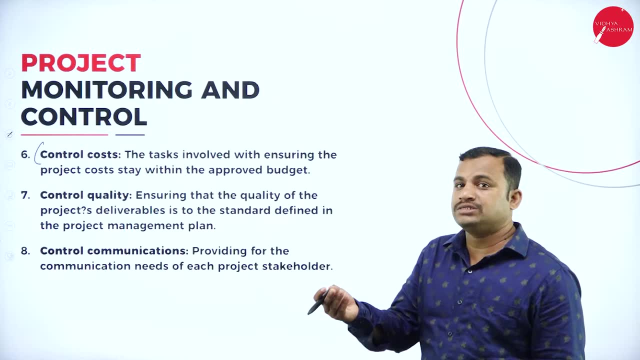 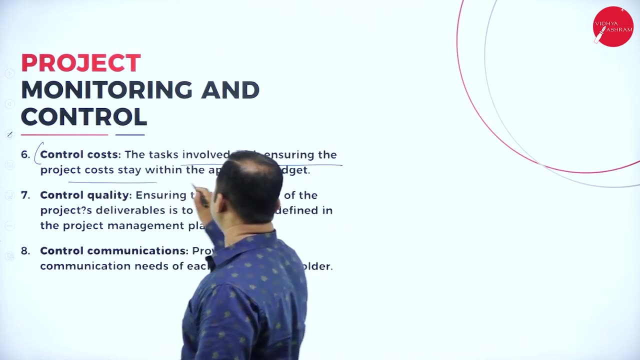 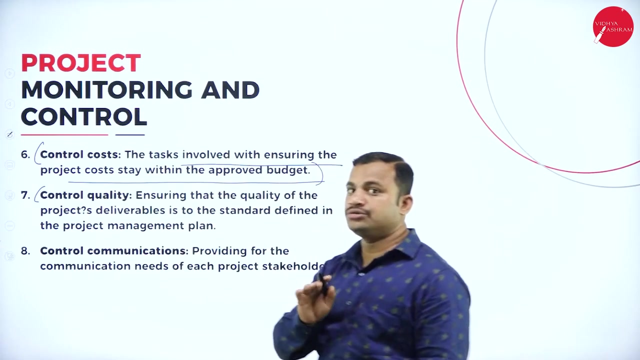 specified time that has to be completed. then control cost: by doing the proper documentation, the cost of that, that is, the expenditure that is incurred for that particular project, can be controlled very well. the tasks involved with ensuring the project costs within the approved budget the same thing. control quality: they have to ensure the quality product to the client, that is. 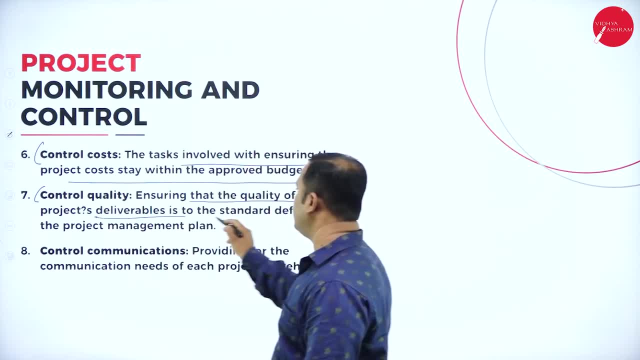 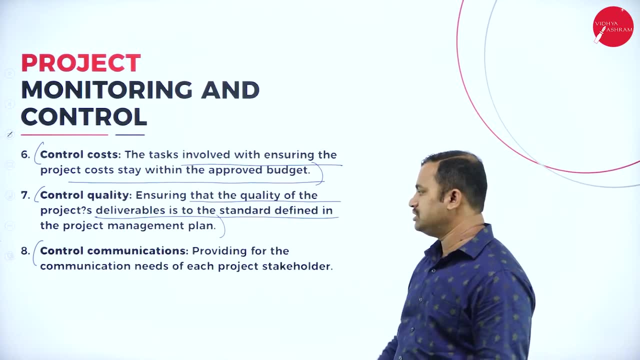 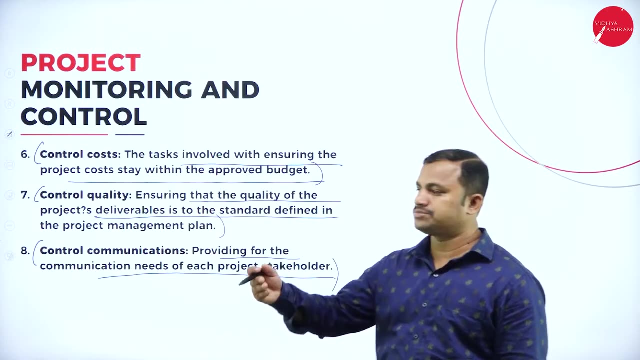 also very, very important: ensuring the quality of the projects deliverables to the standard defined by the project management plan. then control communications. what is the meaning of communications here? the providing for the communication needs of each project stakeholder, how it has to be communicated and explained to. 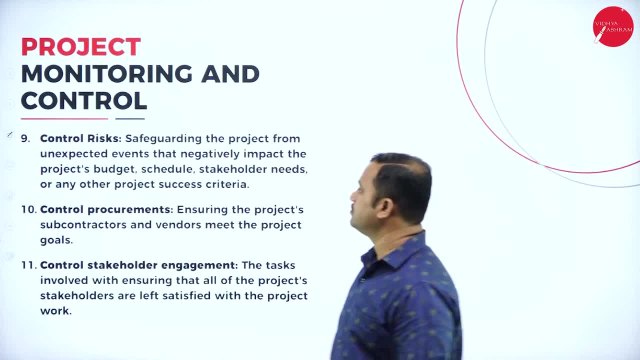 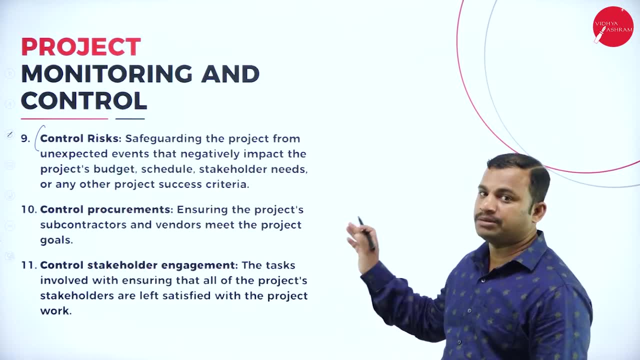 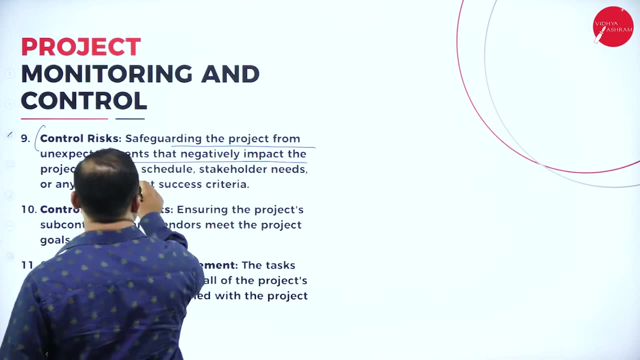 the stakeholders, that is, to the client. control risks: the risks identified at the time of development must be controlled and managed by the project manager as well. that is safeguarding the project from unexpected events that negatively impact the project's budget. because the estimated project management requirements are: attribute it to the eighth under pued status part. 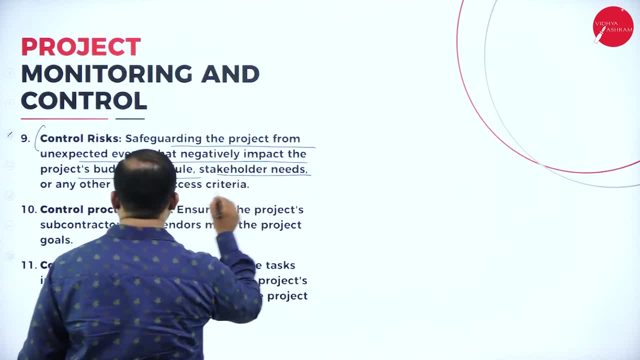 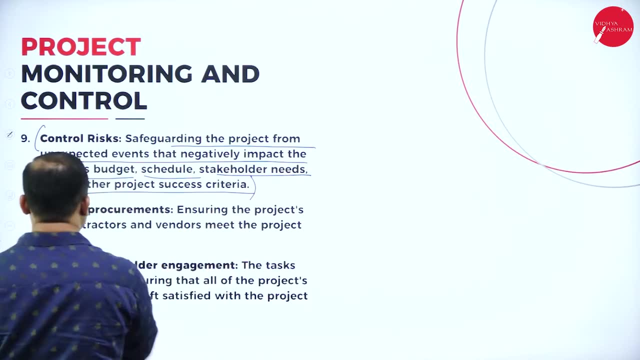 must not be exceeded. So schedule stakeholder needs or any other project success criteria must not be overcome by the team members. Then control procurements. What is the meaning of that? Suppose if there is any technology like the purchased or licensed version. 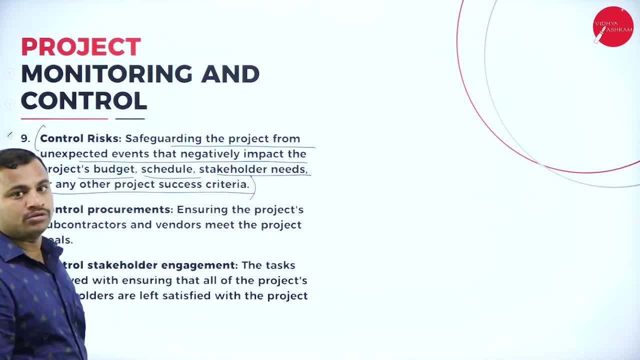 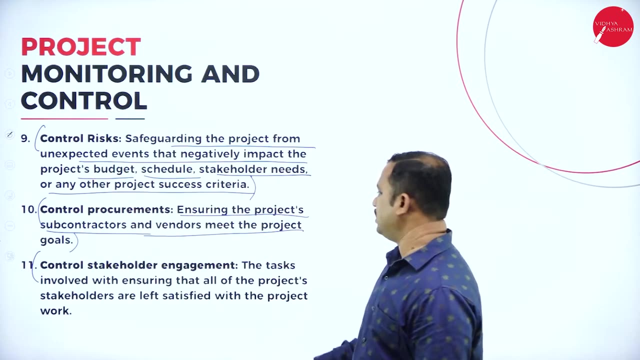 of the software is needed for implementing the code, then it has to be procured. That is, ensuring the project's subcontractors and vendors meet the project goals. How the goal of the project is going to be met with the help of this, Then control stakeholder engagement. 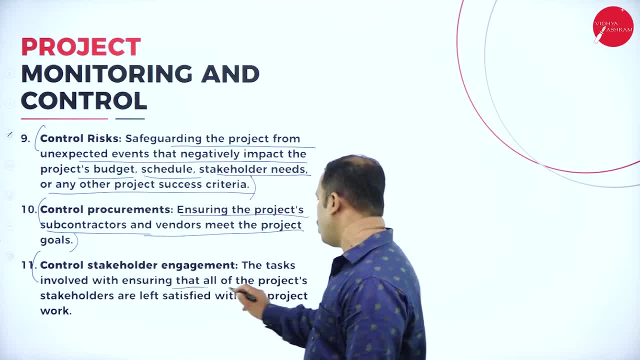 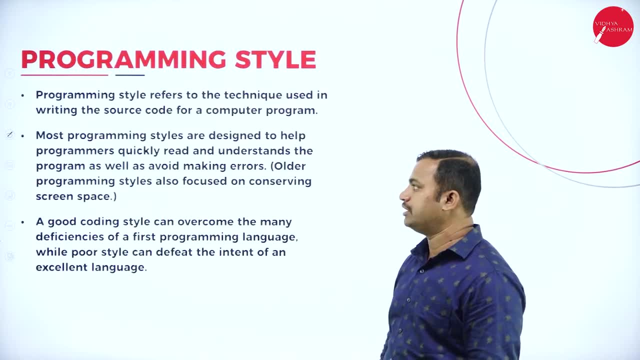 That is, tasks involved with ensuring the quality, That is, all of the projects. stakeholders are left satisfied with the project work, That is, the quality. deliverables are very, very important. Then programming style, which includes the programming style, refers to the technique used in writing the source code for a computer program. 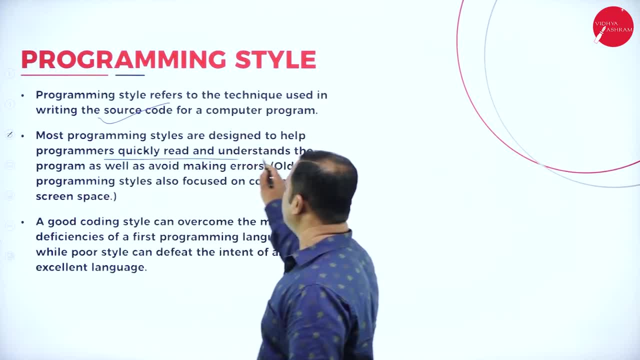 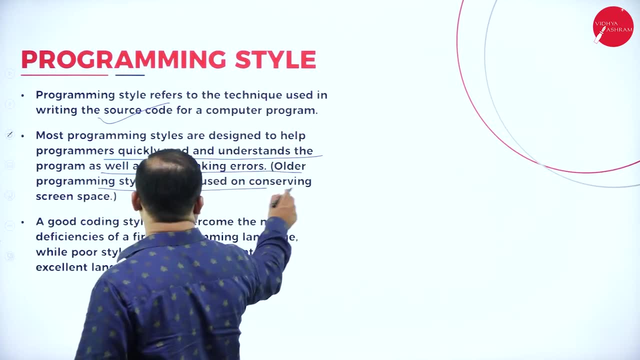 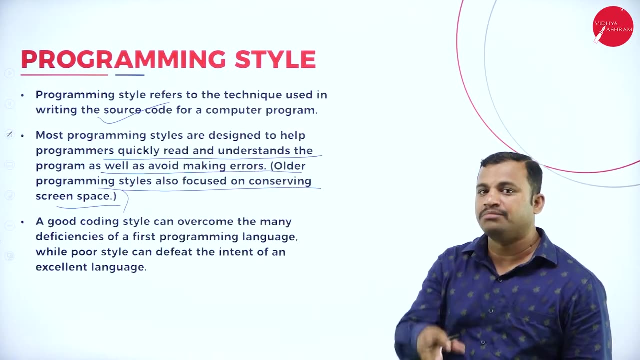 Most programming styles are designed to help programmers quickly read and understand the program, as well as making errors, avoiding the errors. That means older programming styles also focused on conserving screen space. What does this mean? The code written for a particular requirement or to implement a particular task are identified. 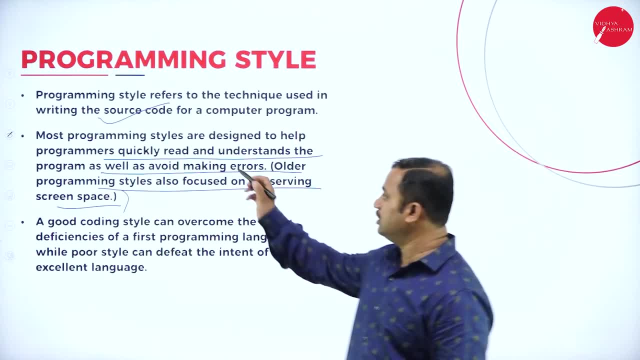 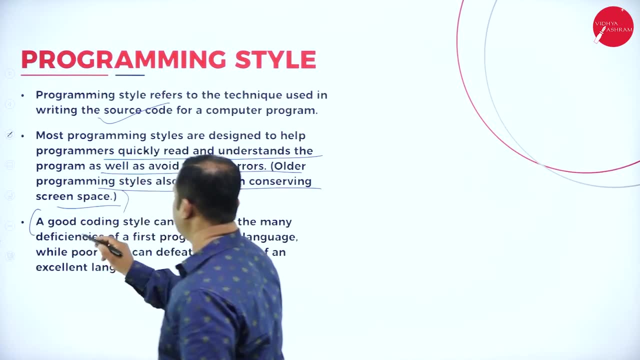 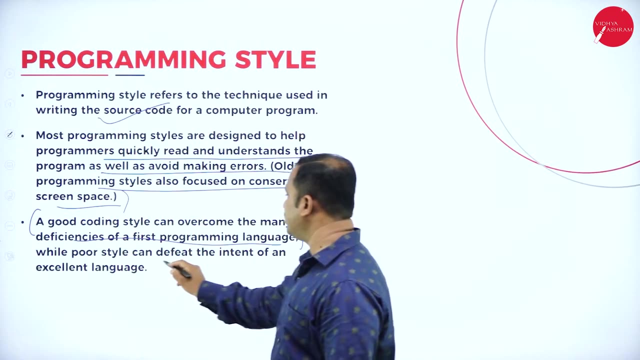 with certain comments, as I have already discussed with you. That is also very, very important and a good programming style- a good condition is a good coding style can overcome the many deficiency of the first programming language. while poor can defeat the intent of an excellent language. 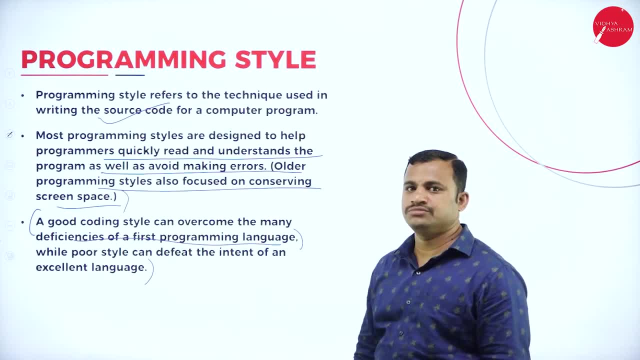 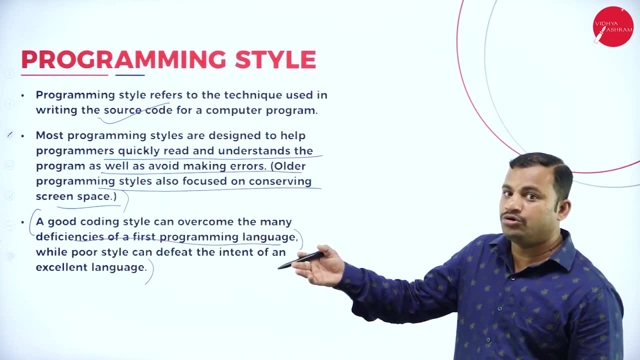 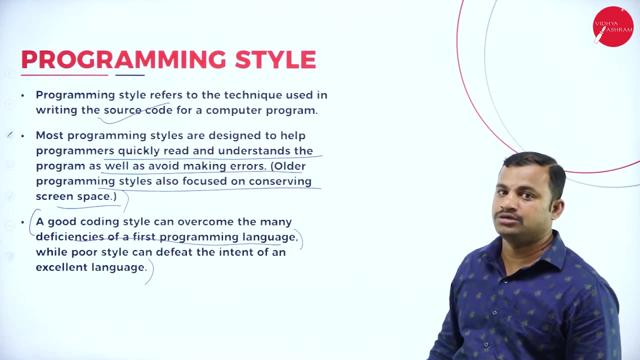 The same thing. When the good coding style is used, obviously that leads to a good product delivery. When there is a poor style of programming, even though it's a good programming language is having the knowledge of that- it is not possible to deliver the software product. 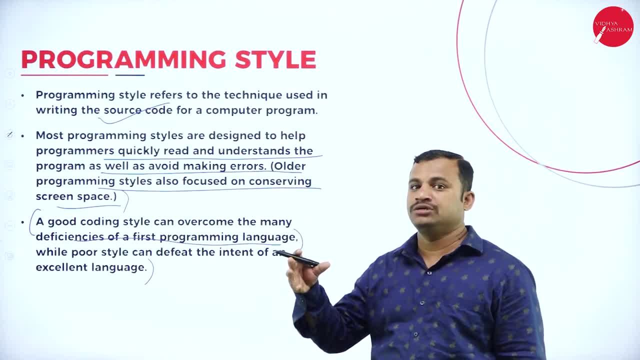 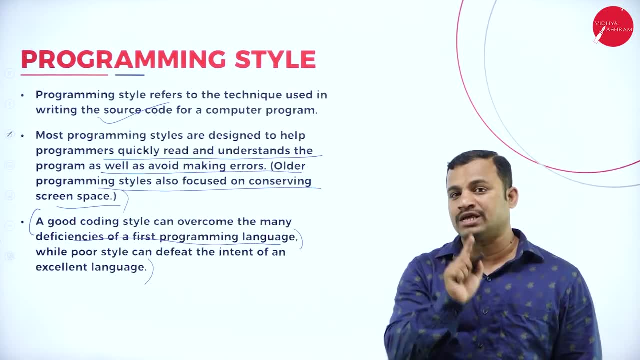 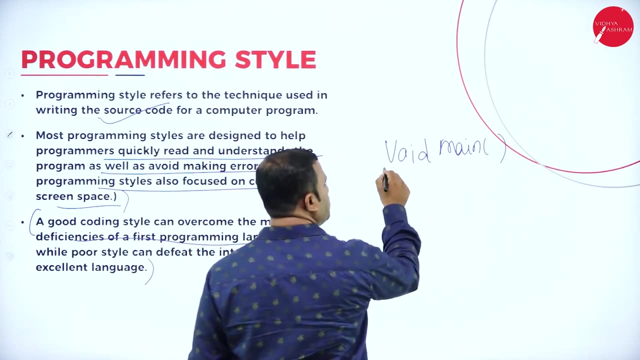 So that is the reason both programming language and the style of programming is very, very important. For example- let me give you one such instance- If I write down any program, I will have to follow them indentation. That is also one of the important programming style. 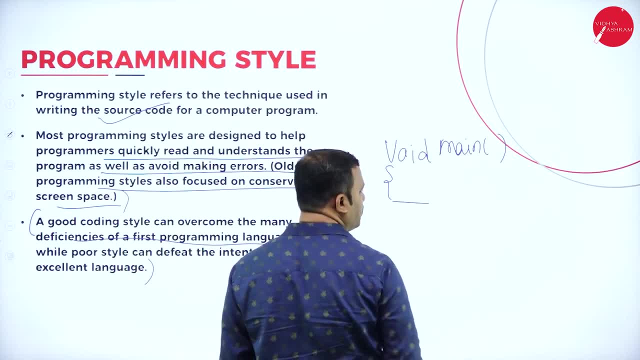 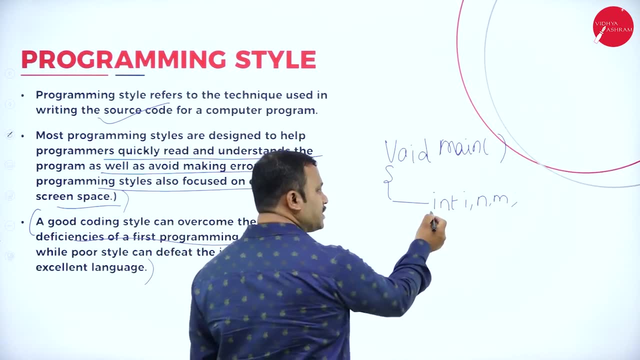 If I started here, the next must be exactly after one tab. I have to follow this: int i n, m, so on like that, Then, which is the next statement that has to begin exactly at the below. So we have to follow this indentation rules. 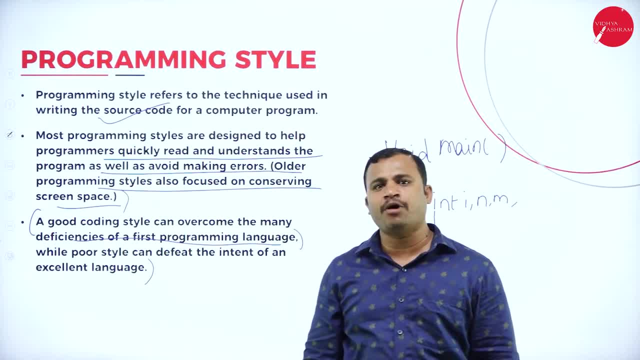 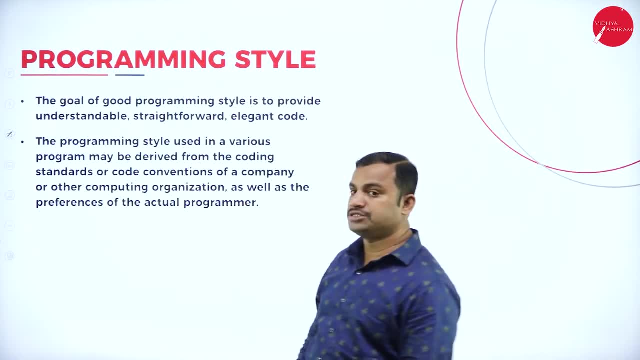 That is the way of programming. The programming style is very, very important in addition to the language knowledge which he has in that. So it is most essential. Programming style plays a very significant role for the developer. The goal of the good programming style 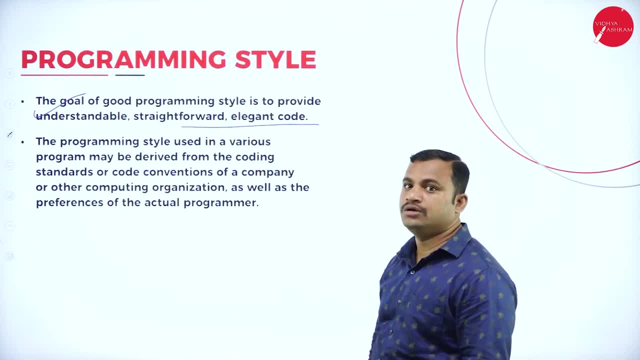 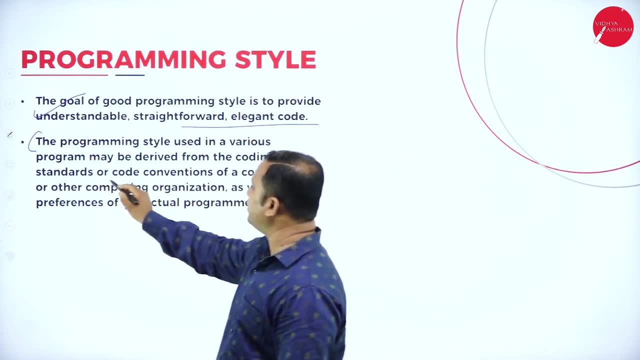 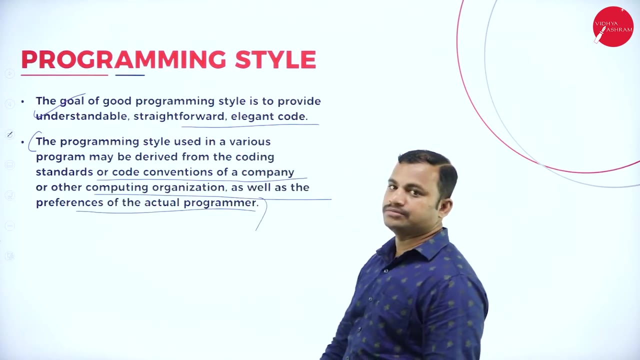 is to provide understandable, straightforward and elegant code, Good coding is required. The programming style used in a various program may be derived from the coding standards or coding conventions of a company or other computing organization, as well as the preferences of the actual programmer. 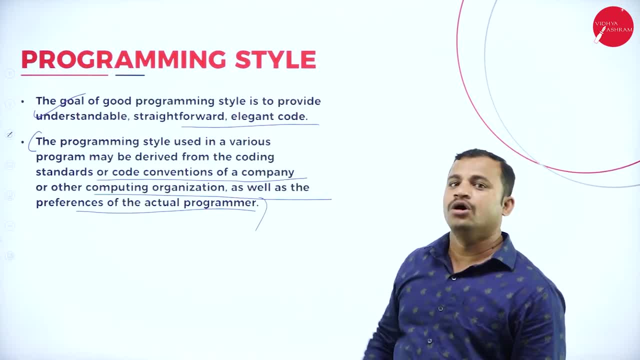 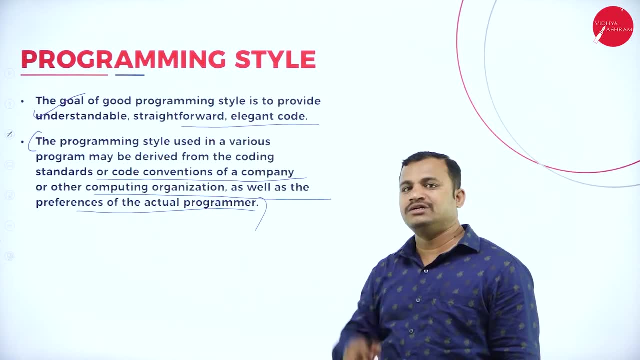 That means that all depends on the coding standards defined by the company. Also, it also depends on the programmer who does the coding, because many of the companies will be having their own coding standards. That means this has to be the logo they have to use in the product. 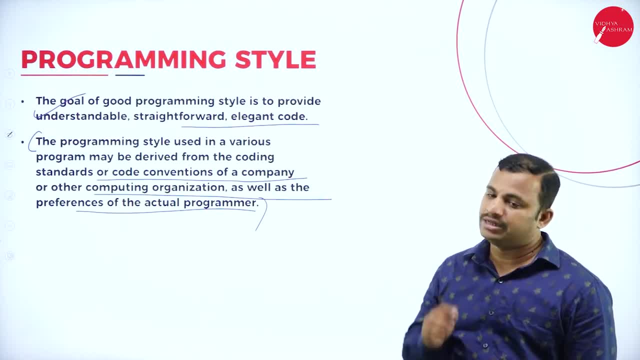 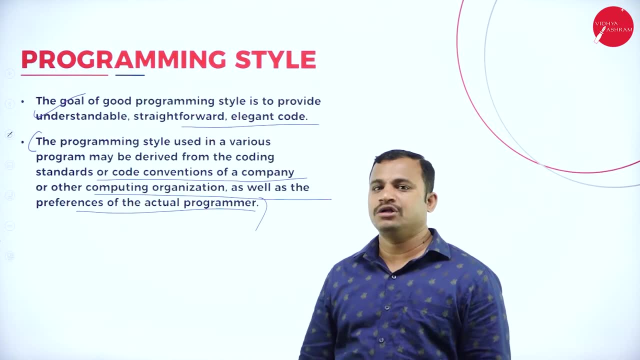 And all those standards are specified, Pre-specified, by the company that has to be incorporated into it, Or else, in some of the companies, it is left to the discretionary information of the programmer who does the task. so with this you will learn that coding guidelines, that is. 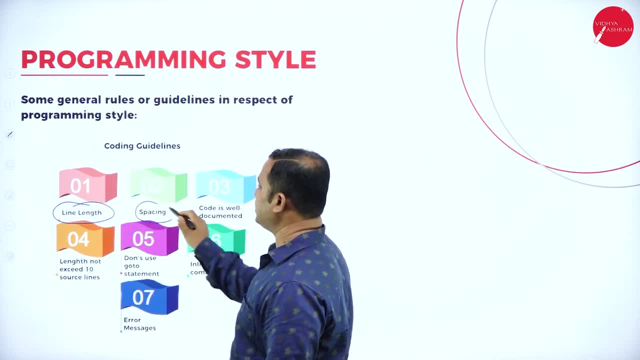 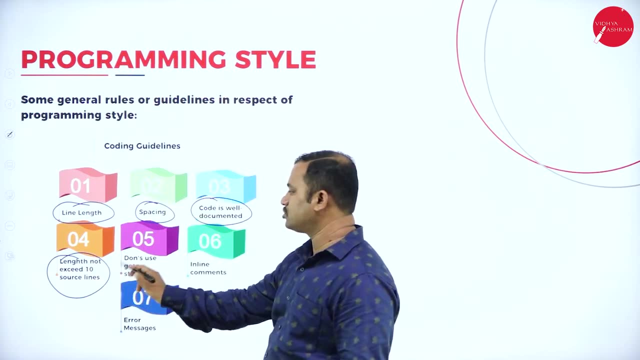 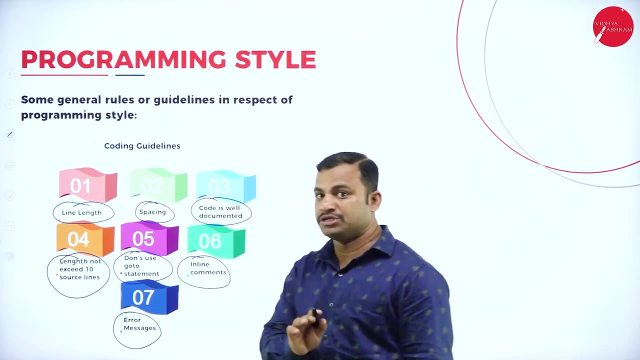 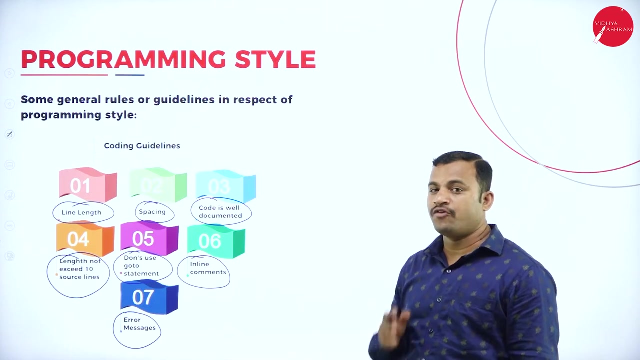 the line length, that is the program length. spacing, indentation, spacing code is well documented or not. then length: not exceed 10 source lines don't use. go to statements, inline command, then error messages, that is, information giving messages. all these are certain guidelines specified, pre-specified by the company, which needs to be followed very carefully by the programmer. 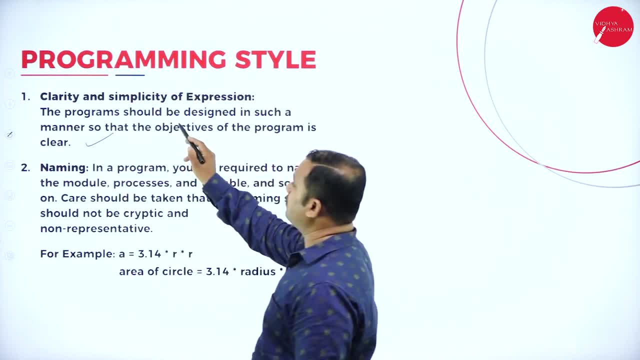 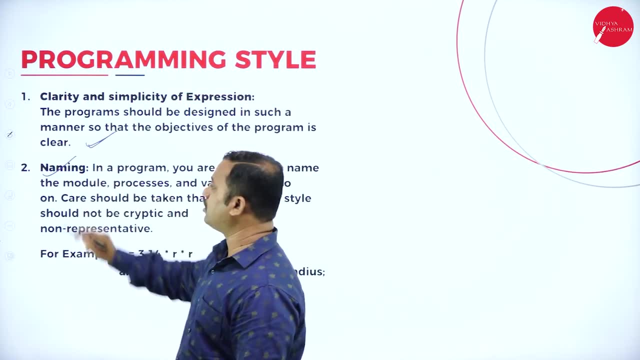 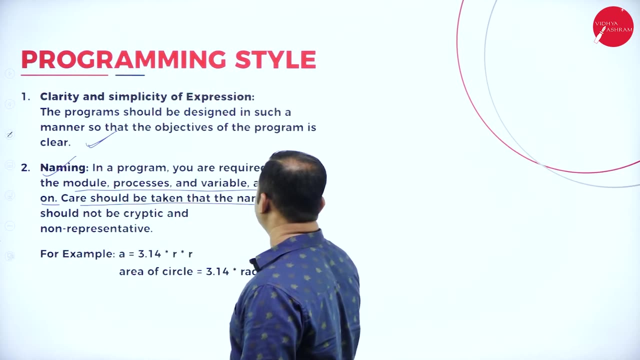 clarity and simplicity of expression. this refers to: the programs should be designed in such a manner so that the objectives of the program is clear. then naming is very, very important. that is, the conventions they use, the modules, processes and variables, and also so on. care should be taken. 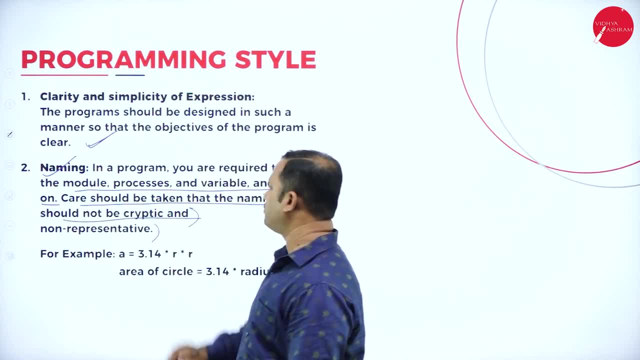 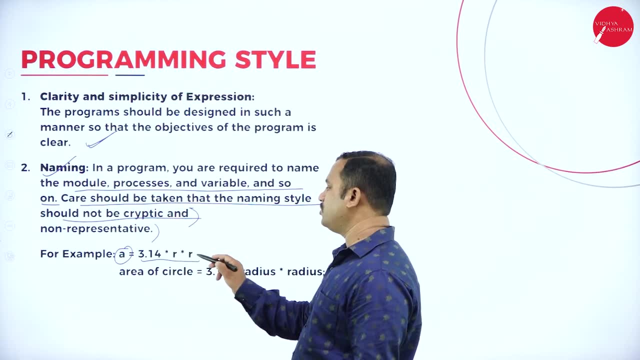 so that the naming style should not be cryptic and non-representative. for example, a is the convention i am using here, 3.1415 into r, into r, where radius to radius. here i am using area of a circle. this is different from this, so naming convention is also very, very important. i am using 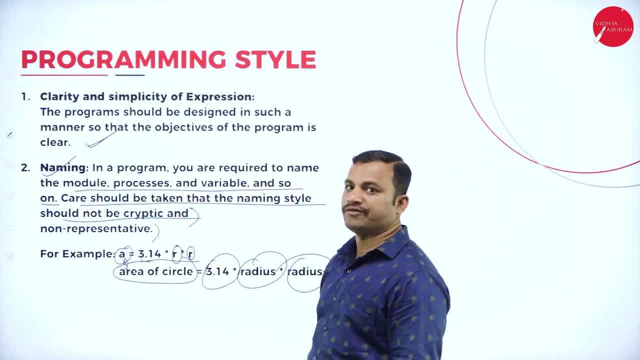 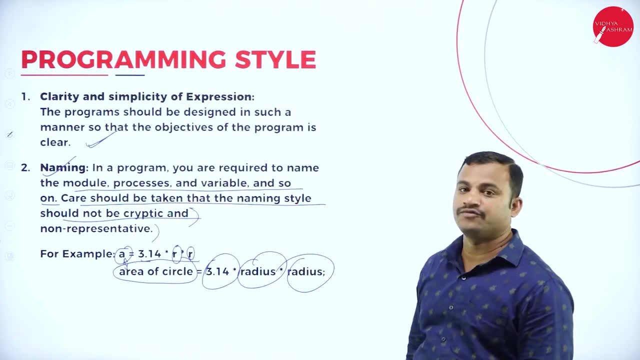 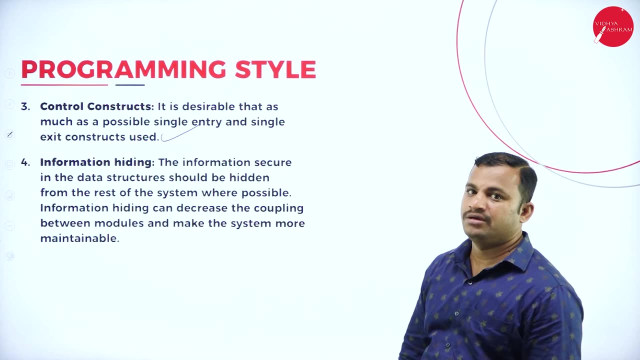 radius here so 3.1415. so that leads to an misinterpretation. so in order to do the interpretation properly, we must have to follow the naming conventions properly, then control constructs, for example entry point and exit point. that is the entry point and exit point. 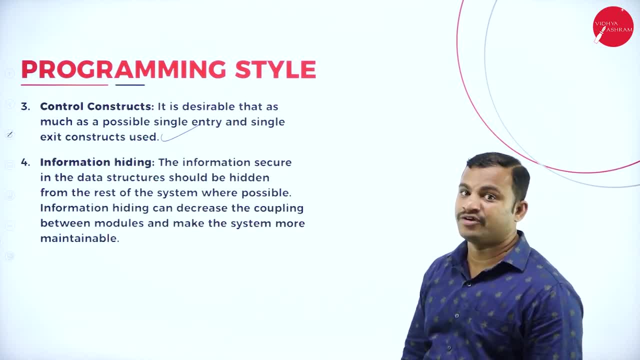 must be defined very carefully using the conditional constructs like if else, if else, if, ladder nested, if all those are certain important type of conditional constructs that place a significant role in it, then information hiding, that is abstraction, that is required. document, document information is given to the user, otherwise the other things are hidden from. 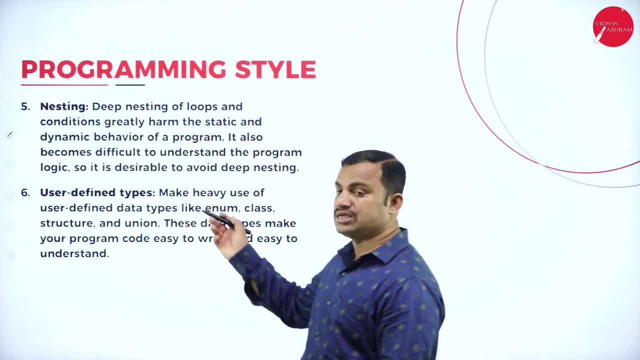 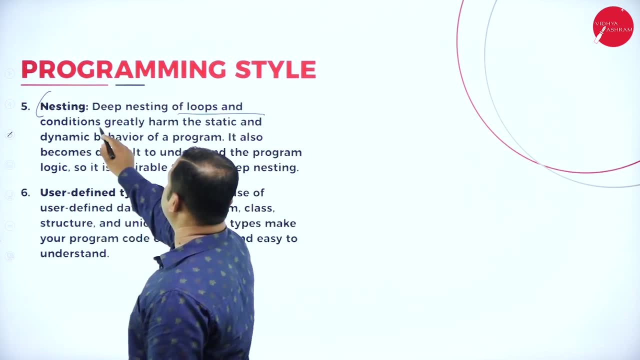 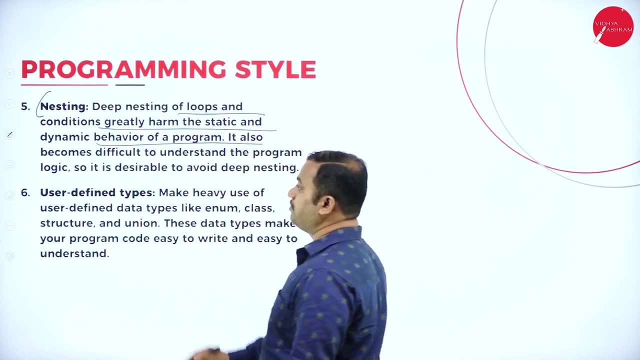 the user. that is called as an information hiding the nesting, as i have already told you, the conditional statements, with nesting one within the other, deep nesting of the program. so, for example, if i want to do a loop and conditions greatly harm the static and dynamic behavior of the program because that increases the time complexity of the program. 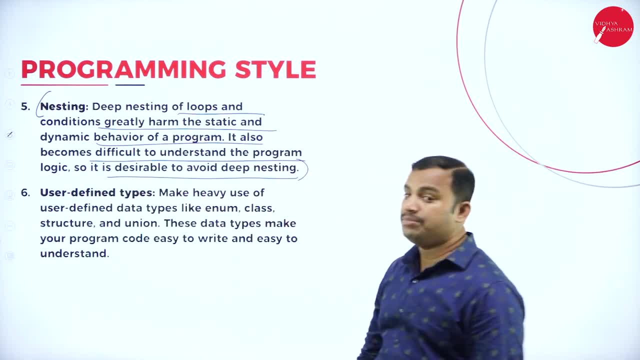 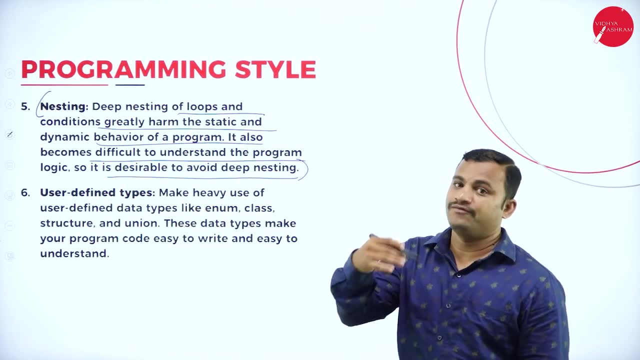 please notice this. it also becomes difficult to understand the program logic. so it is desirable to avoid deep nesting. one logic within another logic, that is, one if statement within another if statement, one for loop within another for loop, one while loop within another file loop. that also increases the time complexity of the execution of a program.